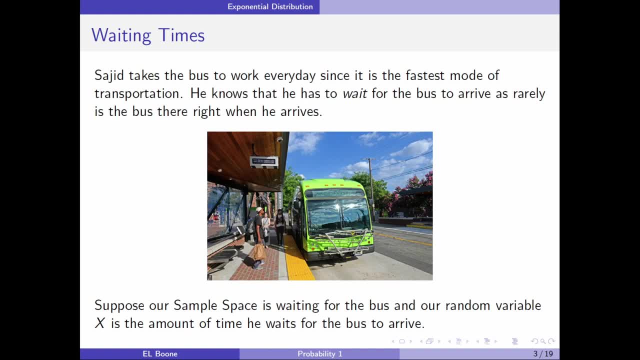 waiting time. So Saja takes the bus to work every day, since it's the quickest way for him to get to work And he knows when he gets there he's going to have to wait for the bus to arrive, as rarely is the bus exactly there when he shows up in the morning or in the evening when he goes home. 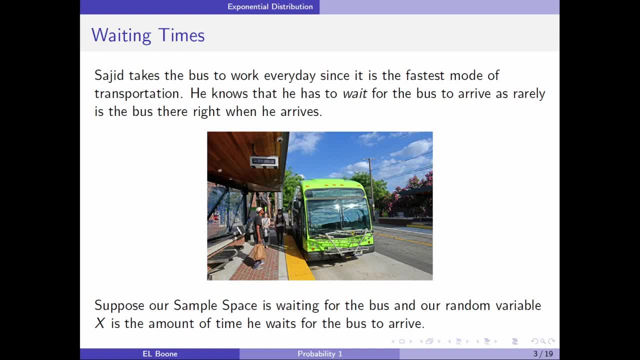 So now our sample space is waiting for the bus. Imagine what that sample space looks like. It doesn't look like an object, It looks like somebody's standing there, which we have right here. Okay, so our random variable here is the amount of time he waits for the bus to arrive. 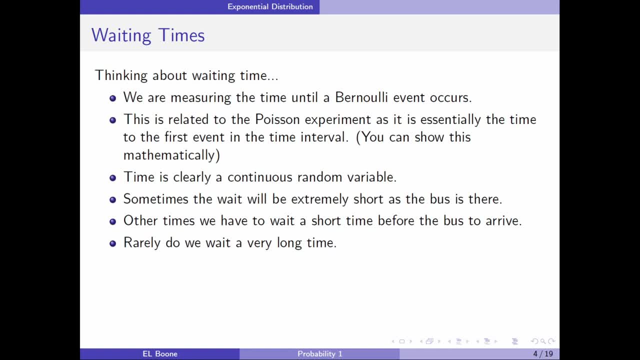 Now let's think about waiting times. Well, we are measuring the time until a Bernoulli event occurs, right? The bus either arrived or didn't, and there's no ambiguity. So this is related to a Poisson experiment, as it is essentially the time to the first event in the time interval, And you 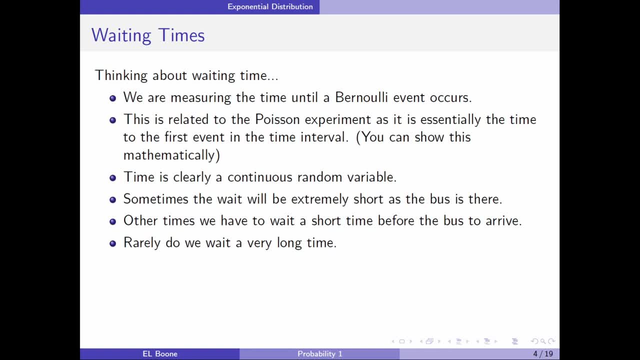 can show this mathematically. We're not going to do that here. Time is clearly a continuous random variable. So we're going to measure the time until a Bernoulli event occurs And we're going to check this out. and again, this is not a brain动". We know that it's to many outcomes to count. 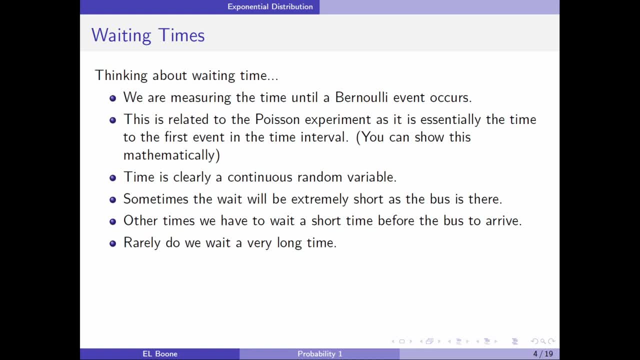 right Milliseconds are involved, so it's clearly continuous Too hard to count, Sometimes where the weight will be extremely short, As the buses pretty much there when you arrive. other times you have to wait a little bit before the bus arrives, And then rarely do we have to wait a. 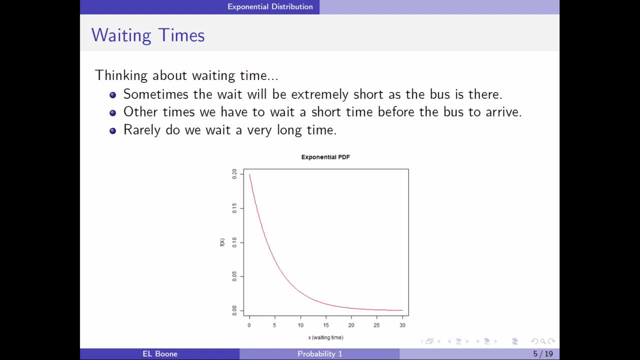 long time. So we think about this. This gives us this sort of shape here. Sometimes the bus will be right there, close, But sometimes you're right there, so close by, But sometimes the bus will be given this particular shape. Sometimes the bus will be right there or close by, And this sort of�entime. 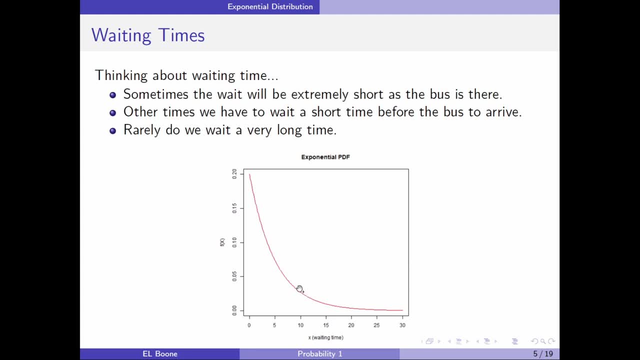 but it takes forever. Okay, but sometimes not. It was the most possible possible change that you should have, But quite often. but then sometimes we have to wait. some notice. this is kind of how likely it is, but long waiting times are extremely rare. right you, it's extremely. 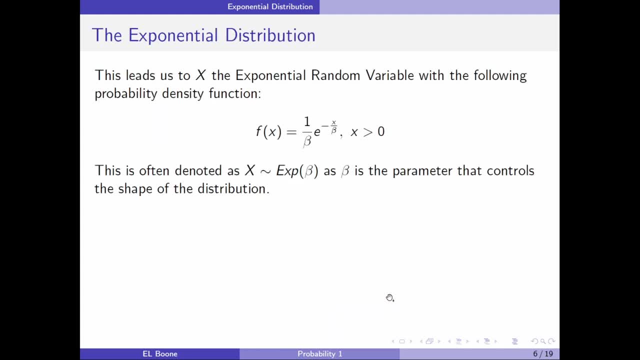 rare, and that's how you think about waiting times. the exponential distribution allows us to do this with an exponential random variable and it has the following probability density function. I didn't make it complete yet. I'll stick that at the end, but often you'll see this written as X is. 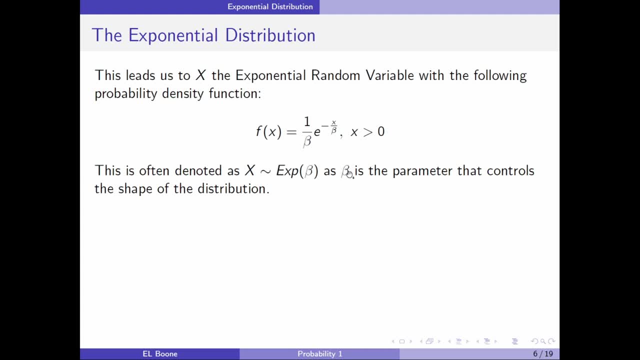 distributed as an exponential, with a parameter, beta, and this beta controls the shape of the distribution and it comes in quite handy, as we will see in a minute. okay, so here's a picture of what it does. so if beta is equal to 2, you can see it's quite likely that there'll be very little waiting time, but it'll be. 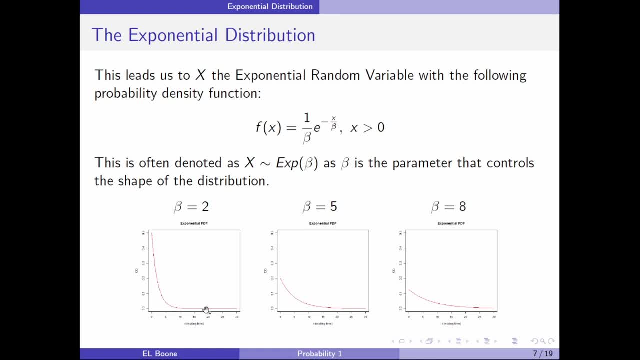 extremely unlikely that you would wait any time more than 10 minutes, where you, if you look at when it's 5, you can see: wow, it's not nearly as likely to be 5, but it's not nearly as likely to be 0, as when beta is equal to, and it's far more likely to have waited 10 minutes. 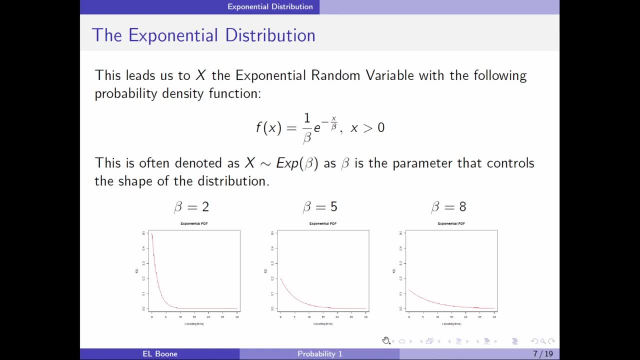 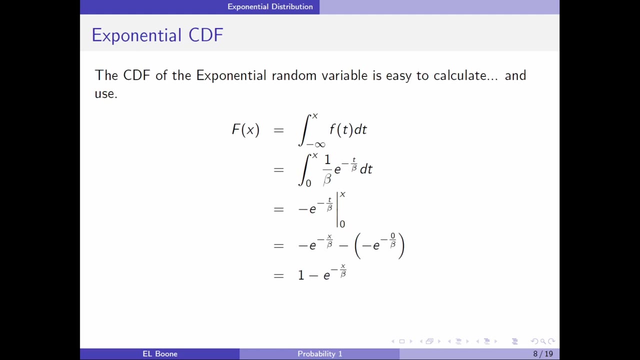 here than 2, and then when beta equals 8, look it gets compressed farther down and gets stretched farther out. more probability is pushed farther out in time. okay, so we can use the CDF, and the CDF here is really really easy to calculate using calculus. so I didn't feel bad showing you if you don't know. 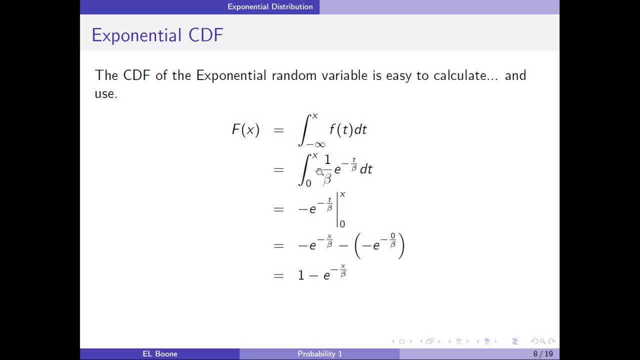 calculus. the answer is at the bottom. okay, so here you just gonna use the definition of the CDF. plug in your density, evaluate it. this integral is really easy. plug everything in 0 and X and you end up here, which is makes us really easy to calculate. this is the formal portion of it. considering: 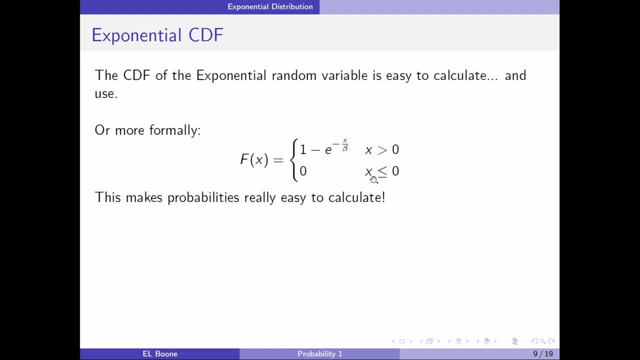 it has the actual 0 involved for when you're less than 0, because nobody waits a negative amount of time. okay, you can show that the mean if you go trace and along here is equal to 1 over beta. we're gonna need this later. this comes in. 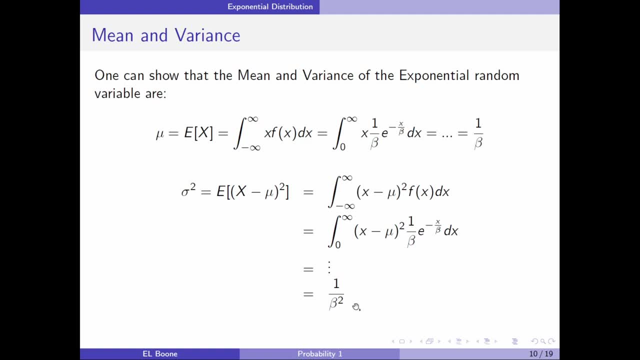 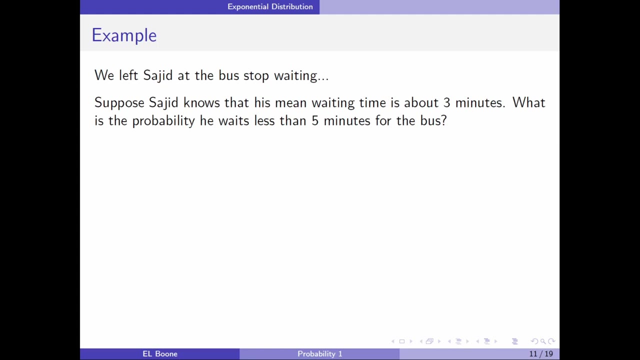 really handy, okay, and that Sigma squared is 1 over beta squared, which is quite handy to have, but we're not gonna really need it today, but keep that in mind for later. all right, so we left Sajid waiting at the bus stop. okay, suppose that Sajid 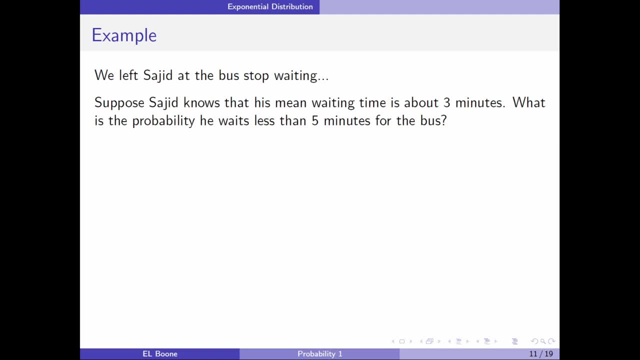 knows that his mean waiting time is about three minutes and he wants to know what is the probability he waits less than five minutes for the bus. okay, it's a reasonable question, okay? well, here's the question: what's the probability he waits less than five minutes for the bus? well, we don't know. 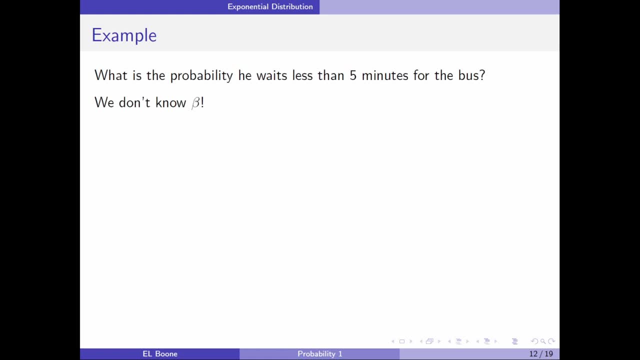 beta. right, because that's that's the thing that controls this distribution and controls the probabilities. well, maybe we do. if we put everything together here, we can see that his mean waiting time is about three minutes. okay, putting this information together, we can. Well, that corresponds to: mu equals 3, and we know that mu is equal to 1 over beta. 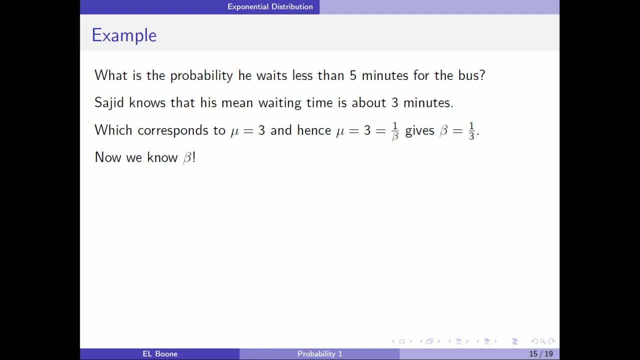 So by solving it for beta, we get that beta is equal to one-third. So we do know beta. It's just it's not directly a number that you can read out of there. You have to think about it for a minute and think about what you know. 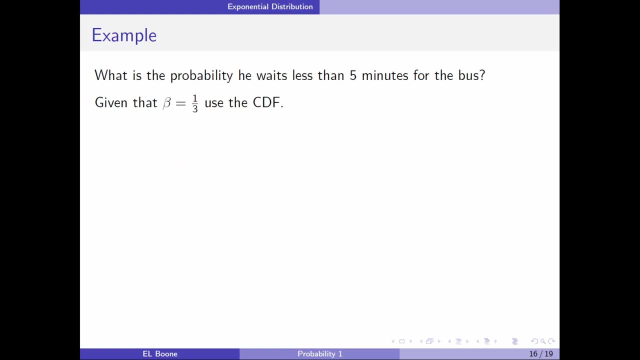 and sure enough, we have the information. Given the probability is less than five minutes for the bus. well, that's a direct use of the CDF. Given that beta is equal to one-third, we just use the CDF, plug in the numbers, which is really easy, right. 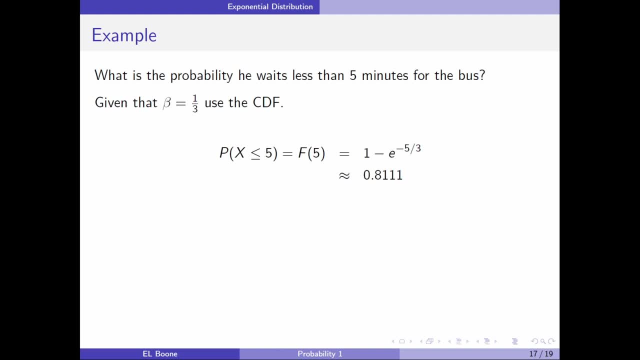 Probability x is less than five is equal to f of five, which is the CDF, which is one minus e to the negative five-thirds. Plug that in your handy-dandy calculator and you will end up with 0.8111.. 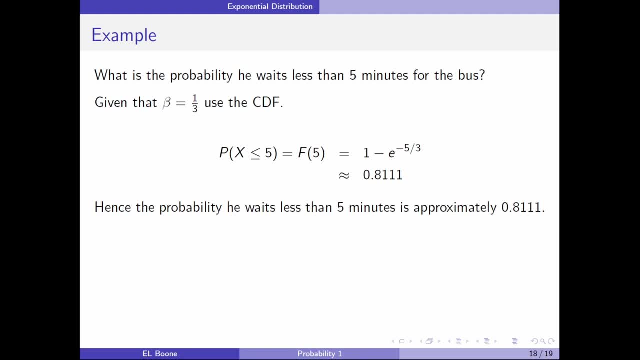 So the probability he waits less than five minutes is approximately 0.8111.. So It's quite likely he's going to wait less than five minutes for the bus, So hopefully he's not incredibly impatient. All right, so quick list of items here. 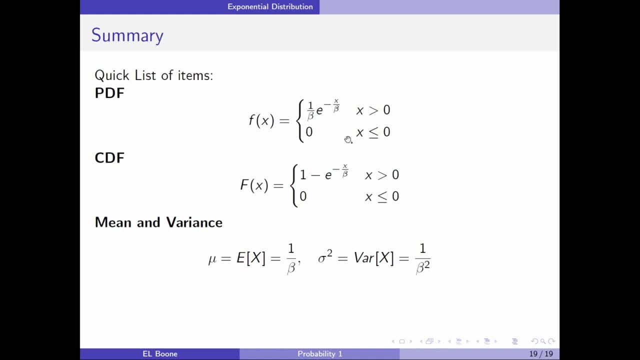 The PDF. is this in its formal version, right? It has the cases here It talks about when it's valid, when it's not valid. Here's the CDF which we've already written in the formal version. The mean and variance of this thing is one over beta. 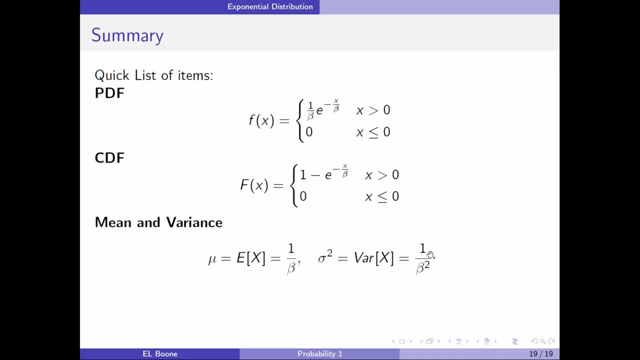 and that comes in real handy, as we've seen, And the variance is one over beta squared, which we'll worry about later when we talk about other distributions. So we're on to the next distribution in the next video. See you there.